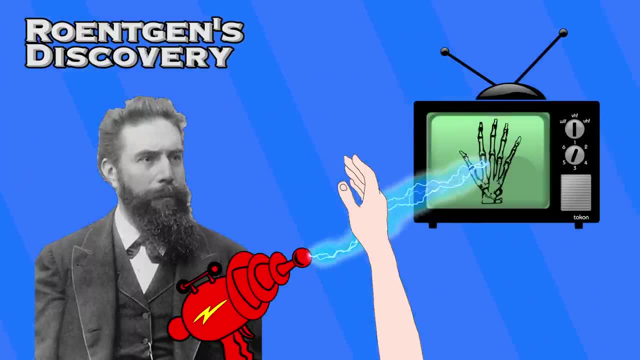 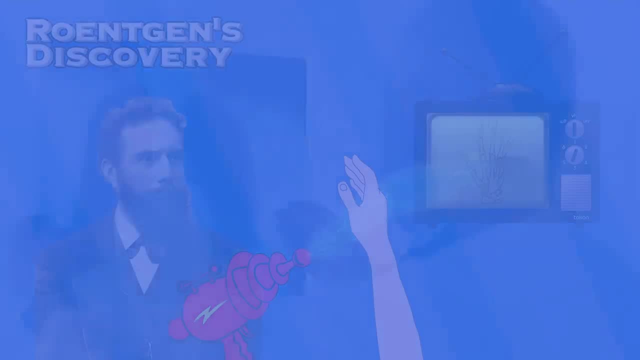 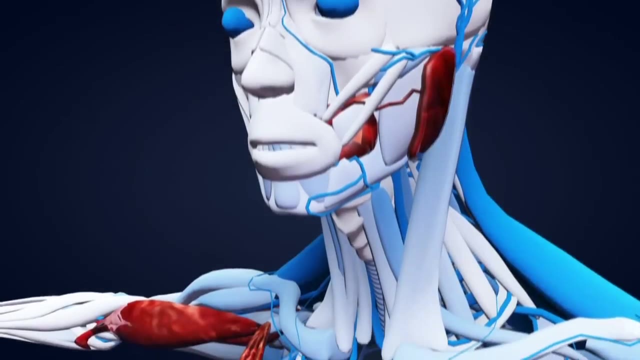 This created an image of the bones inside his hands on the screen, revealing x-rays' perfect use. This double discovery marked arguably one of the most important medical advances in all of human history. It gave professionals the ability to see ailments inside of the human body without 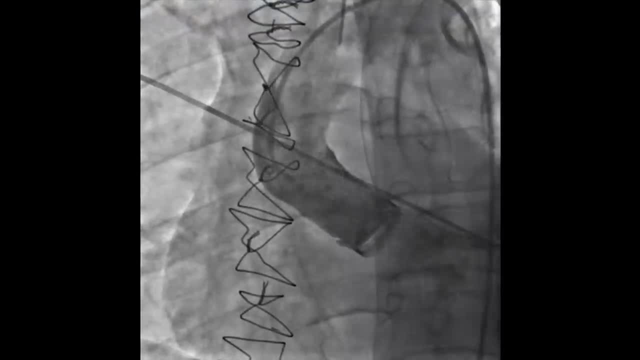 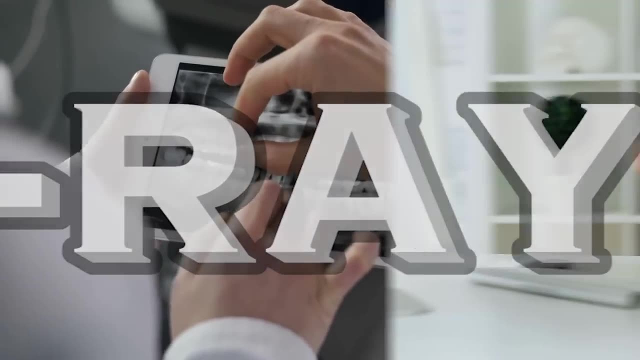 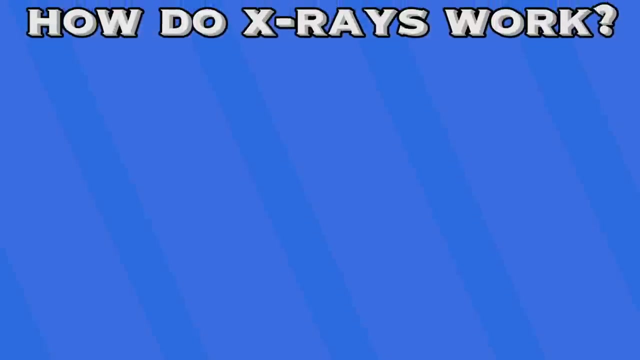 invasive surgery. It even allowed them to see soft tissues, with slight modification. No one questions that x-rays are important to modern medicine, but most people don't have a great idea of what is actually happening when you use them. When you get one, you can think of x-rays as light rays. Both are electromagnetic energy. 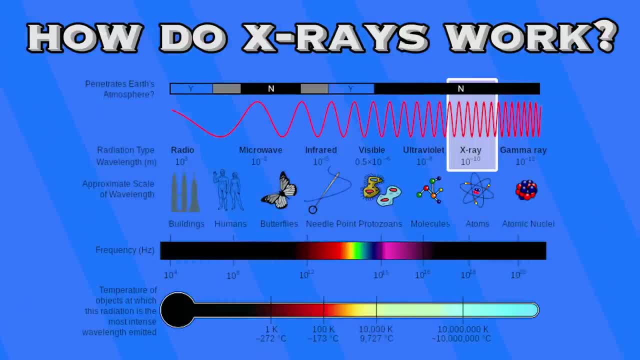 carried in waves by photons. The major difference between these types of rays is the energy level, or wavelength of the rays. We, as humans, have the ability to sense light rays in the wavelengths of visible light, but shorter and longer wavelengths fall outside of our visible spectrum. 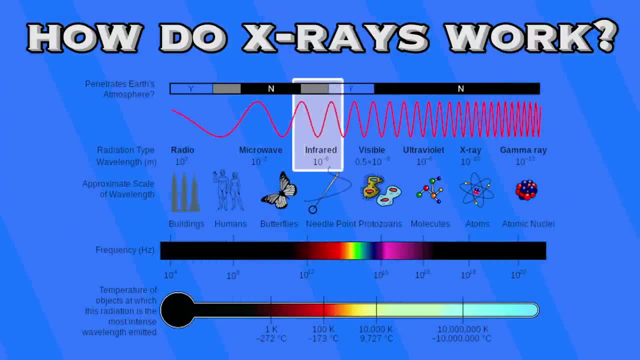 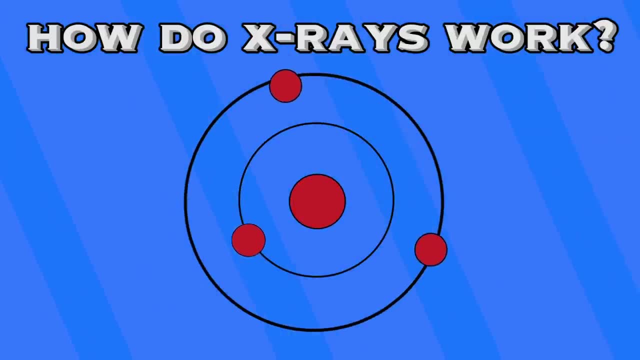 X-rays are shorter. higher energy waves and radio waves are shorter. higher energy waves are longer. lower energy waves- X-rays are produced by the movement of electrons within atoms. The specific energy level of a given x-ray is dependent upon how far the electron dropped. 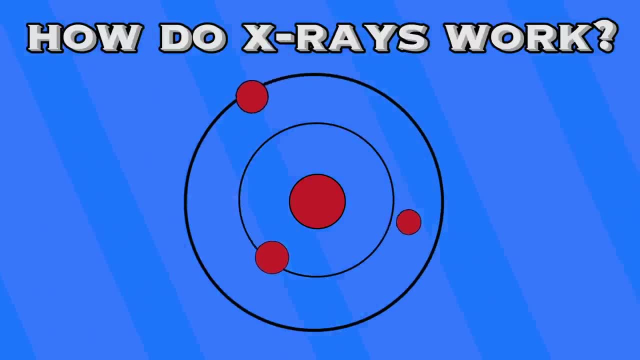 between orbitals in an atom. When any given photon collides with another atom, the atom can absorb the photon's energy and boost an electron to a greater level. In this case, the energy of the photon has to match the energy difference between the two electrons. 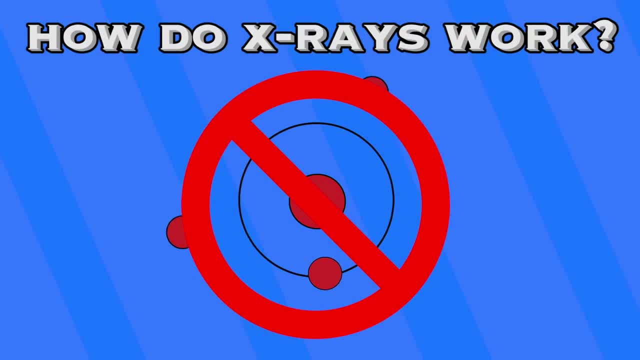 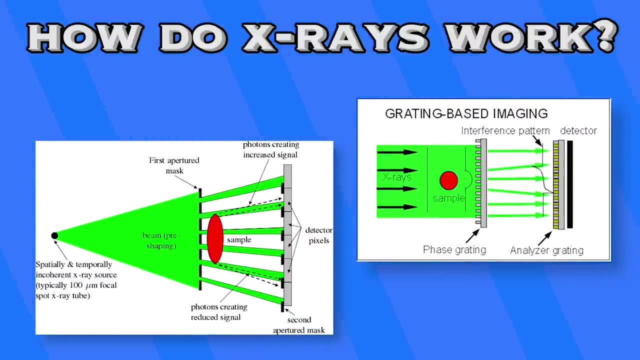 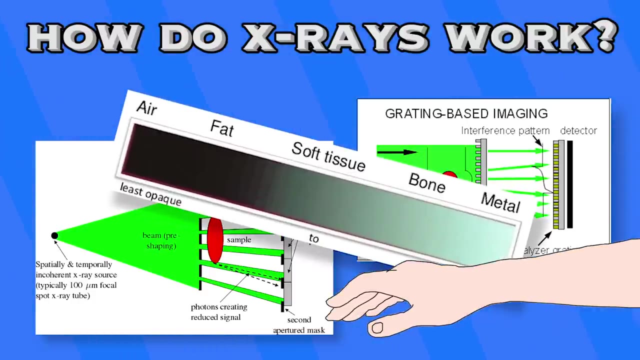 If this doesn't occur, then the photon can't cause a shift between orbitals. This functionality means that as photons from x-rays pass through your body, each tissue's atoms absorb or react to photons differently. The soft tissues in your body are composed of smaller atoms, so they don't absorb x-rays well due to the photon's high energy. 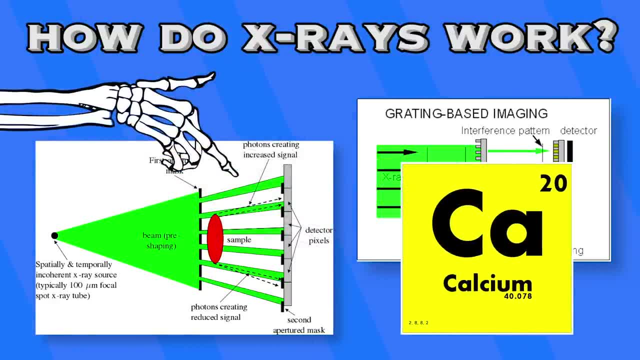 On the other hand, the calcium atoms of bones are much larger, so they do absorb the x-ray photons and thus result in a different future. The x-ray photons absorb the x-ray photons and thus result in a different future. The x-ray photons absorb the x-ray photons and thus result in a different future. 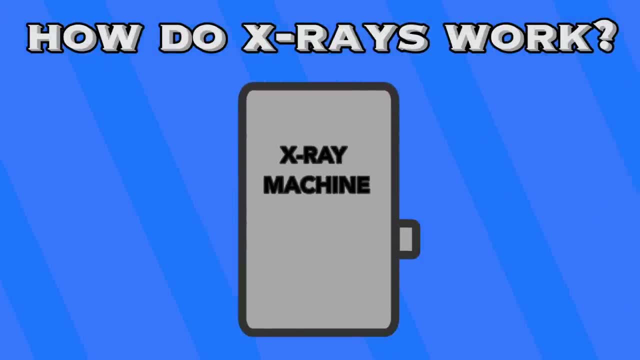 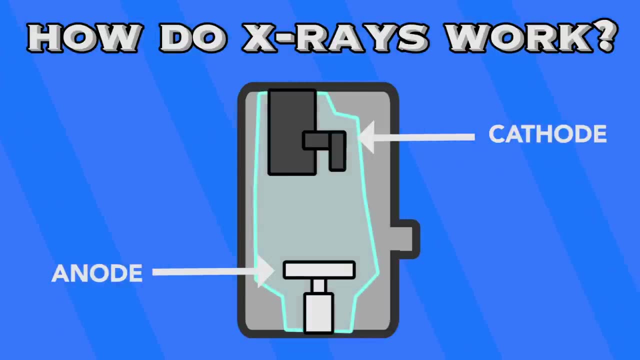 On the x-ray image. inside of x-ray machines there's an electrode pair, an anode and a cathode. inside of a vacuum tube usually made of glass, The cathode is usually a heated filament and the anode is a flat disk made of tungsten. As the cathode is heated up, 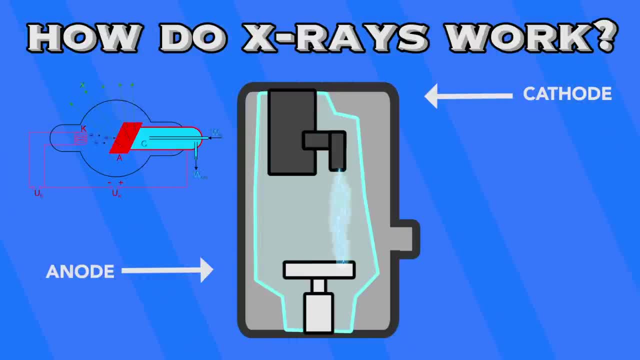 electrons spurt out of the filament and find their way to the anode. The voltage difference between the anode and the cathode is very high, which allows the electrons to travel through the air with a high velocity. As these electrons travel through the tube at such a high pace and 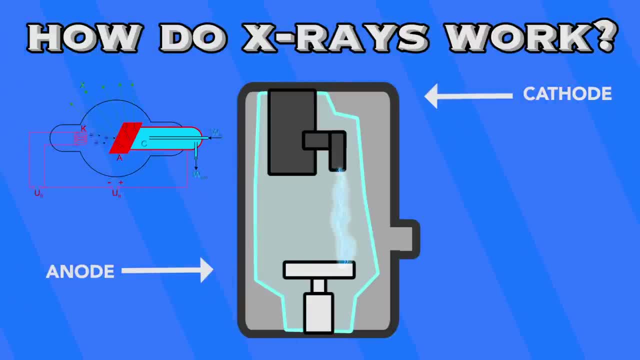 hit the tungsten atoms of the anode. it knocks loose electrons in the lower orbitals of the atoms. As electrons fall from higher orbitals to these lower energy levels, the extra energy is released as a photon. Since this drop is large, it releases high energy photons or an x-ray. 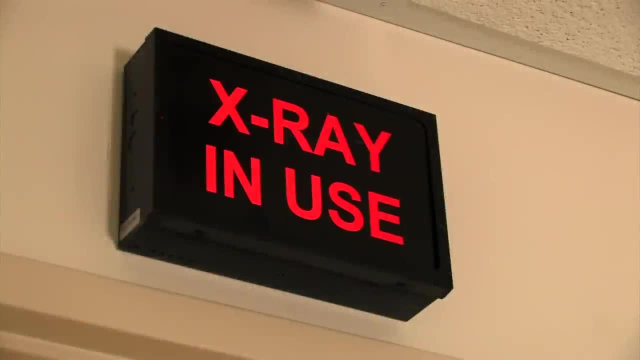 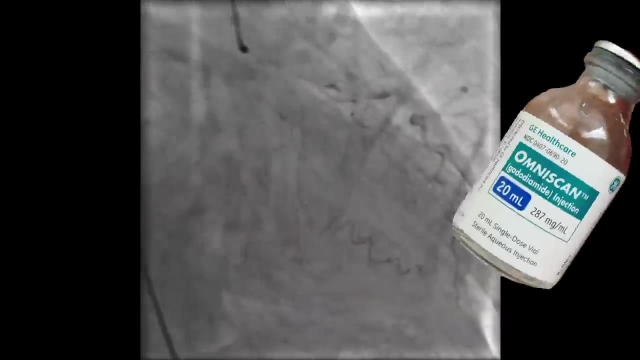 This is how normal x-rays are produced in function, but in cases where soft tissue, like human organs, need to be examined, then contrast media needs to be added. Contrast media are typically liquids that absorb x-rays and collect in soft tissues. 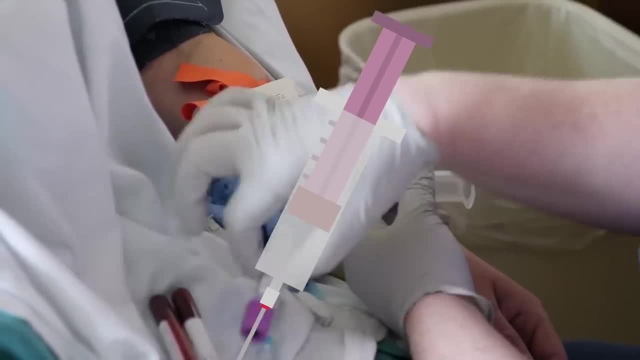 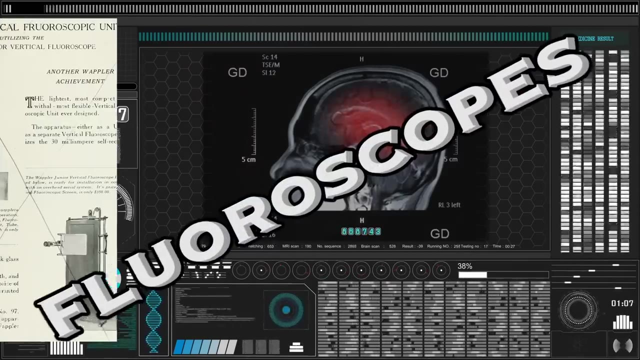 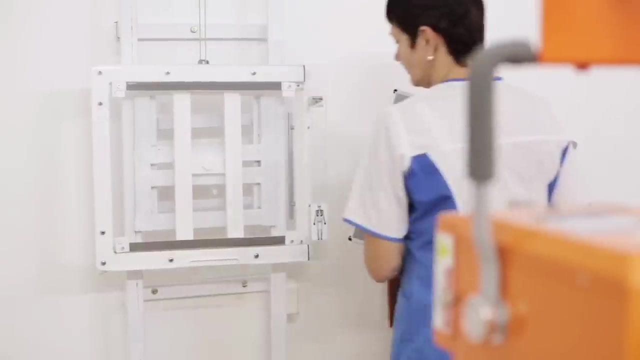 To examine blood vessels, doctors will inject this media into veins. Oftentimes, in these cases of soft tissue viewing, doctors will also use fluoroscopes to see the image in real time and can even capture videos using these devices To collect the actual image. 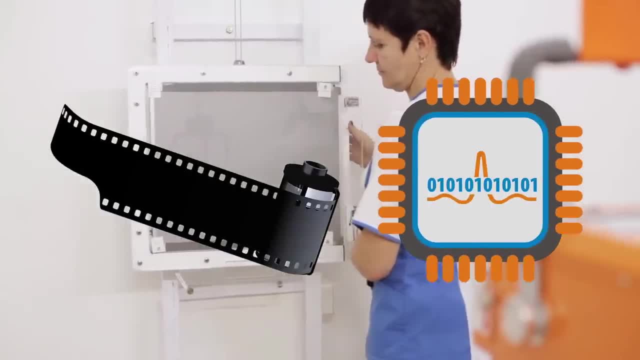 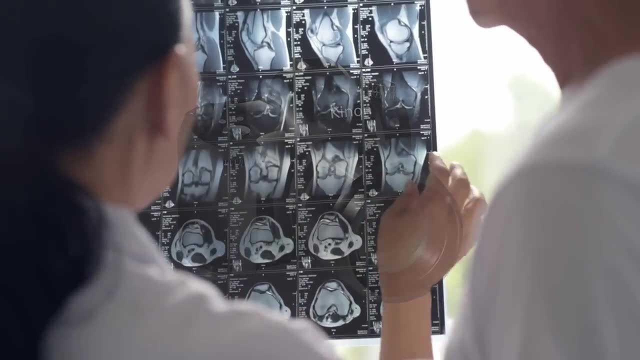 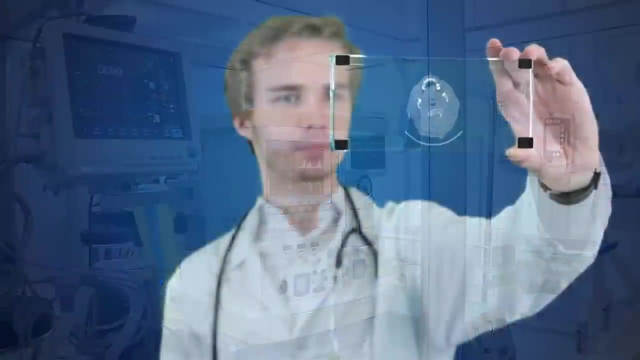 doctors will then use a film or sensor on the other side of the patient. These films work nearly identically to normal photographic film and the sensors are particularly sensitive to x-rays. Through all of this imaging, doctors can deduce a wide array of important medical data from 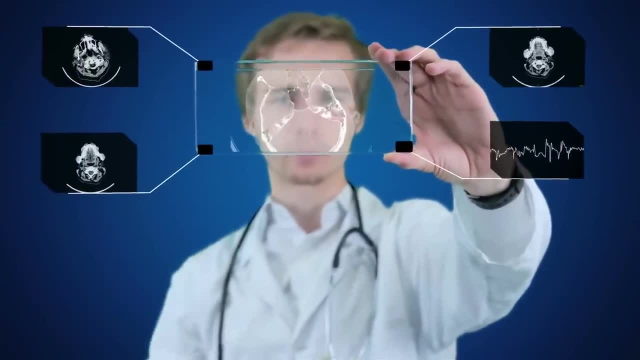 x-rays, And so, even with the significance of x-rays, they can still be dangerous in high doses, as they are a form ionizing radiation. This means that when an x-ray is used, it will pictures present with a whole array of important medical data, and the x-ray can collect a wide array of data. This means that when an x-ray is used, it will create a photographic picture of the patient, and the x-ray also carries the image of the patient. So doctors can deduce a wide array of important medical data from x-rays. To make this imagining, doctors can also use this imaging to detect if an x-ray is.